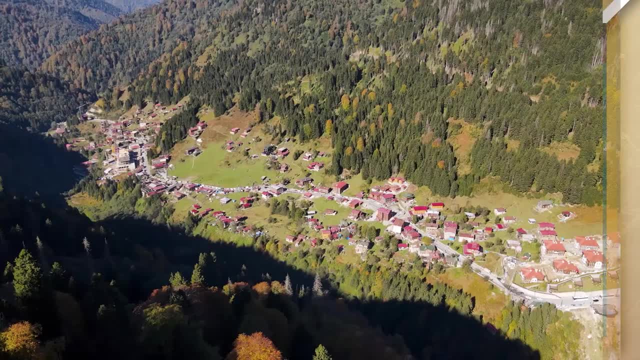 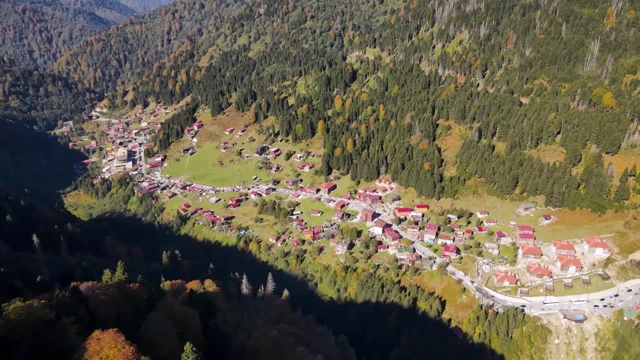 settlements and farms stretch along a main road. In fact, traditionally linear settlements and farms developed along a road, river or some form of transportation system which allows people to quickly get goods and services in and out of the settlement. So now that we've talked about 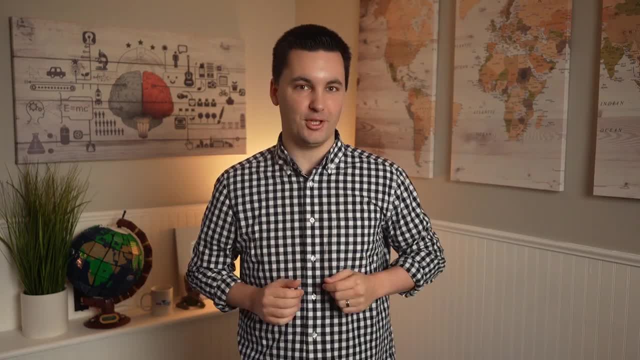 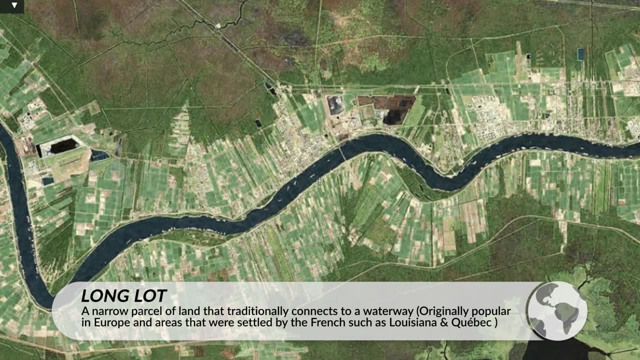 settlement patterns. let's change gears and switch to survey methods. To start, I want to go back to our linear settlement pattern, which here we can also see an example of the long lot survey method. This is when land is divided up into narrow parcels which, each parcel of land having access. 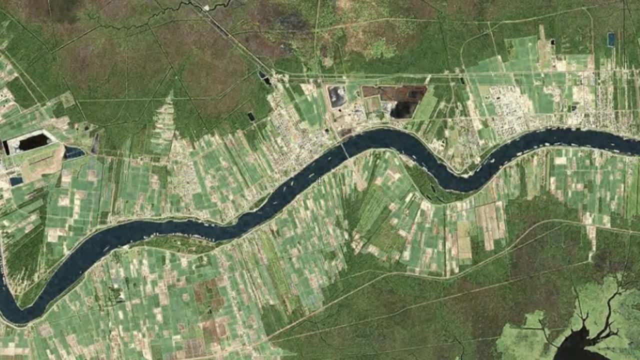 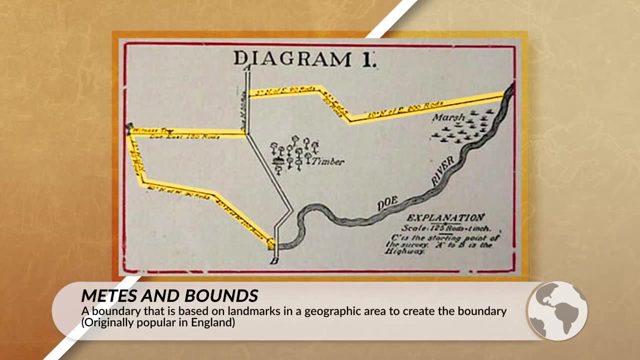 to either a river or a major road, in order for each parcel of land to have access to transportation. Up here we have meets and bounds. Meets are often straight lines that connect different parts of a geographic area, where the bounds are key geographic features that define an area. This 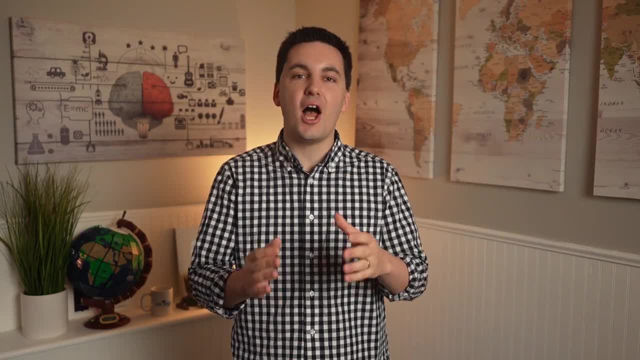 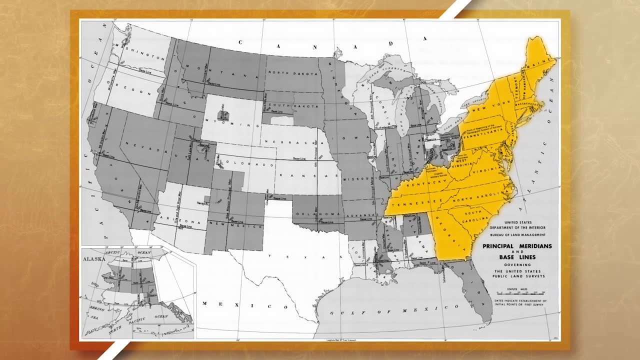 survey method is often used for short distances and relies on key features of a place. In the United States we find meets and bounds used more frequently on the east coast of the United States, where Europeans first settled, with the rest of the country using more township and range as a survey. 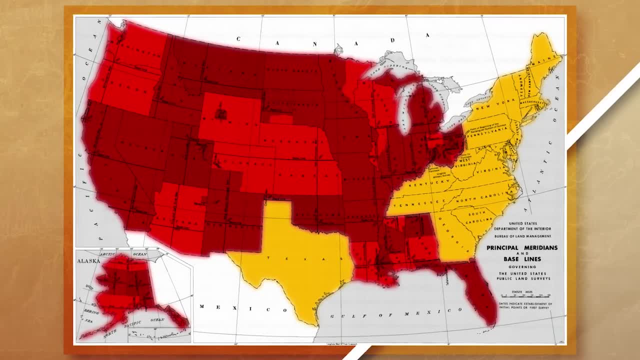 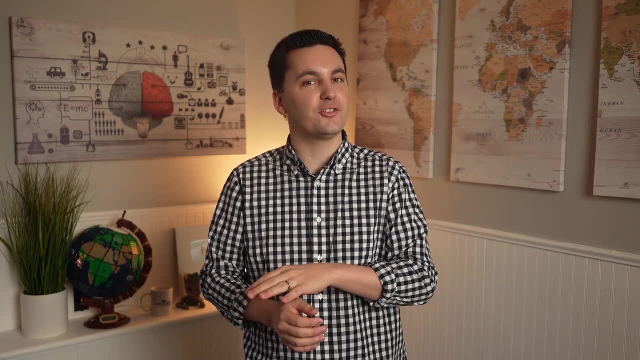 method, with the exception of Texas, which was not part of the United States until later and was more by Spanish and Mexican rules, causing Texas to use more meets and bounds as a survey method compared to the rest of the country that use township and range, which we can see when we move. 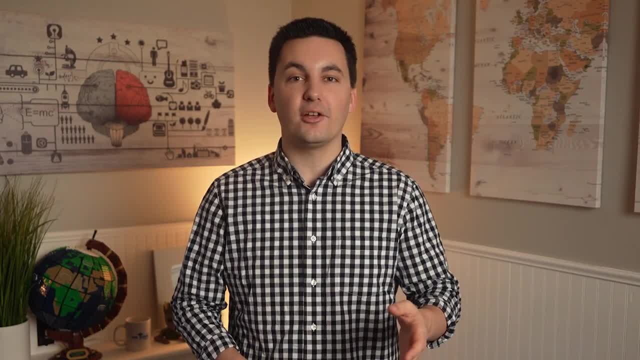 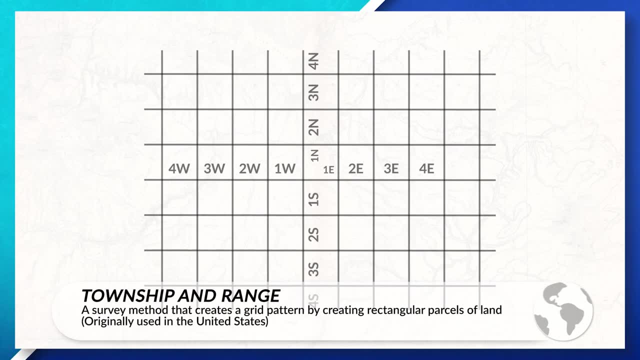 west from the east coast of the United States and move into the midwest and western part of the country where we start to see township and range as the main survey method. When looking at township and range survey method, we will use a baseline, with townships going north to south on the baseline. 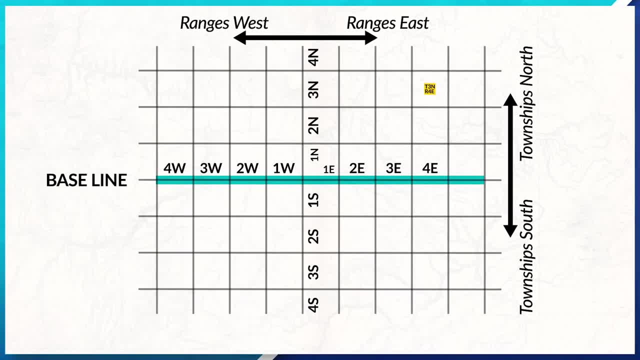 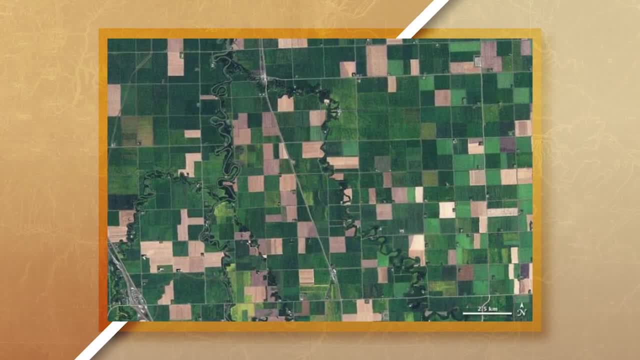 and range going west to east. This survey method uses longitude and latitude to create a grid system. This is a lot more organized compared to meets and bounds and creates clear and distinct pieces of land. This organization makes it easy for people to clearly identify who owns what land. 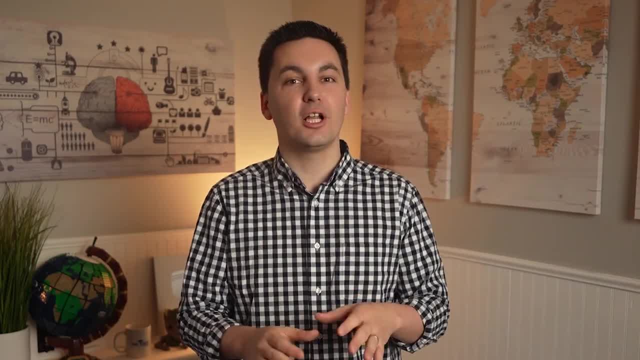 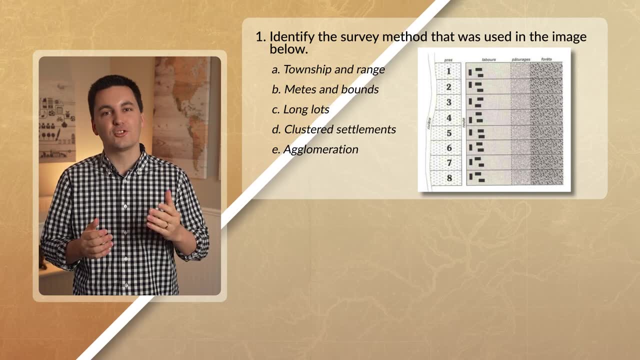 which makes it easier to sell and manage the land, which is important, especially for a country with a large population And just like that. geographers. another topic: review video is done. now comes the time to practice what we have learned. answer the questions on the screen and, when you're done, check.